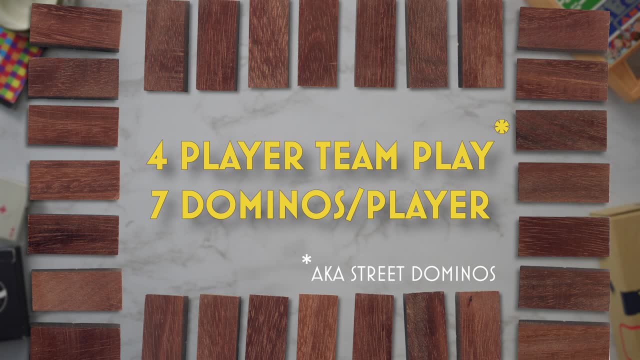 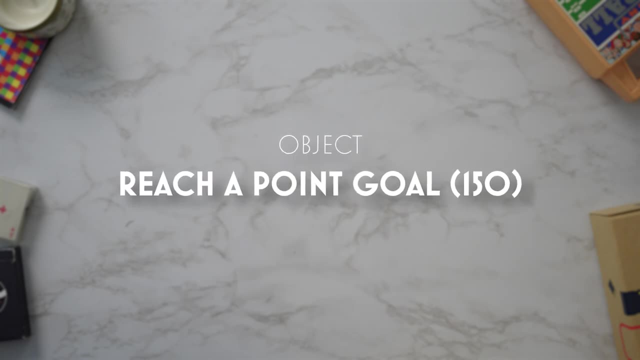 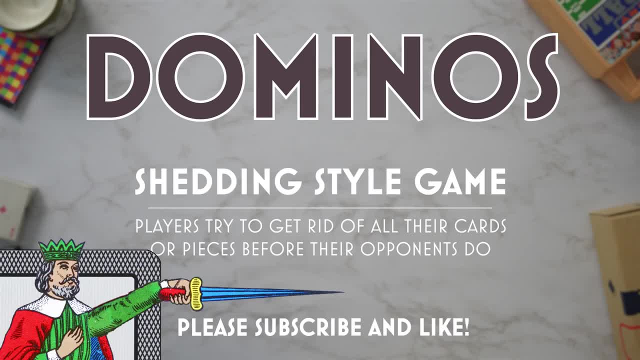 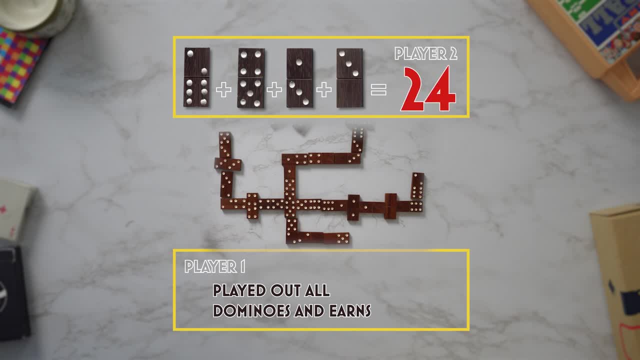 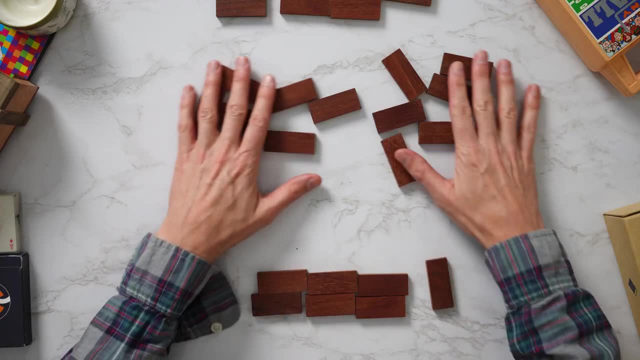 but rather you add up the remaining domino values in your opponent's hands and you get to keep that score. Today we're going to set up a two-player game. Each player is given seven dominoes and the remaining 14 go in a face-down pile known as the bone yard. Yes, the bone yard. Why bone yard? 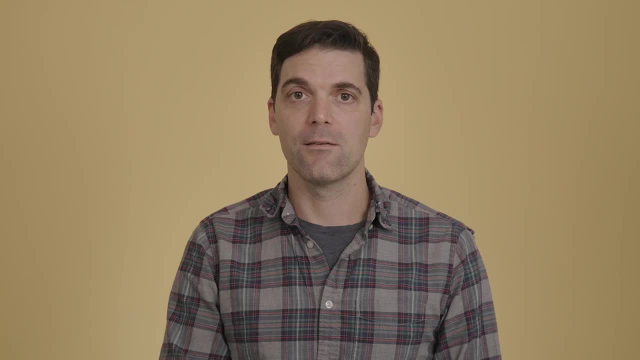 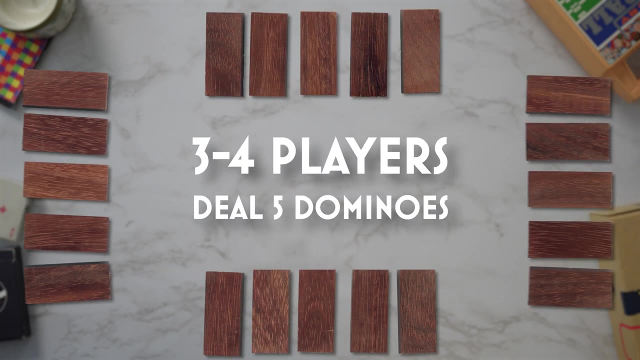 Well, dominoes were originally made with bones and, uh, you put them in a yard. Basic dominoes is best played with two players, but you can play with three or four. Just start each player with five dominoes instead of seven. That said, competitive street dominoes is best. 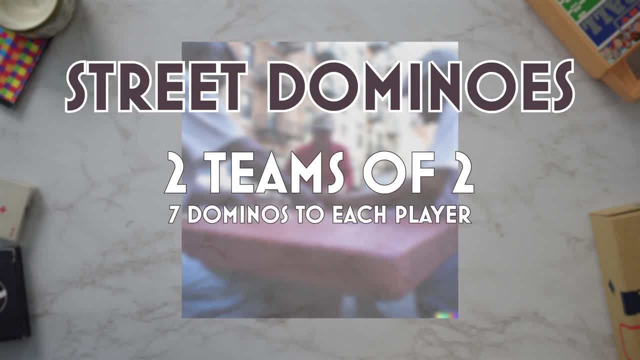 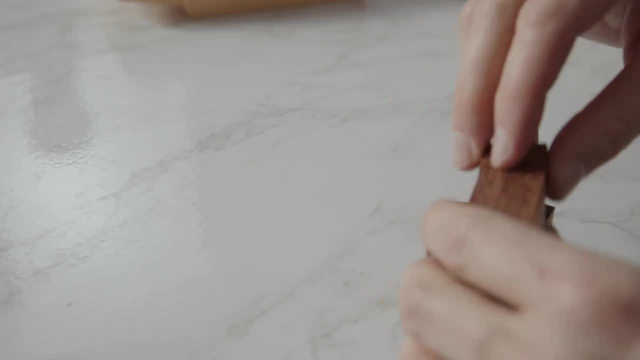 played with four players in two teams of two, Each player getting seven dominoes and a bottle of bergal. No, you're not ready for that yet. Your dominoes are only visible to you. like this, You can stand them up with ways or advanced dominoes. players can hold all seven in their hands like a. 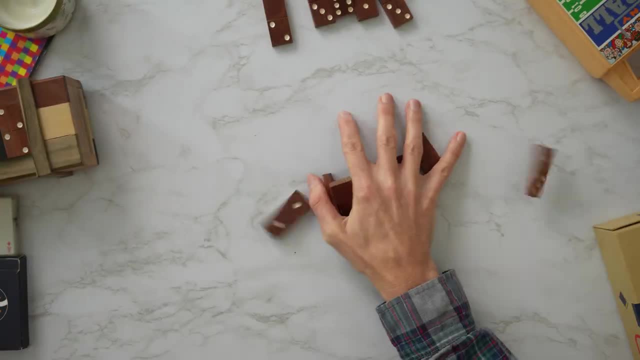 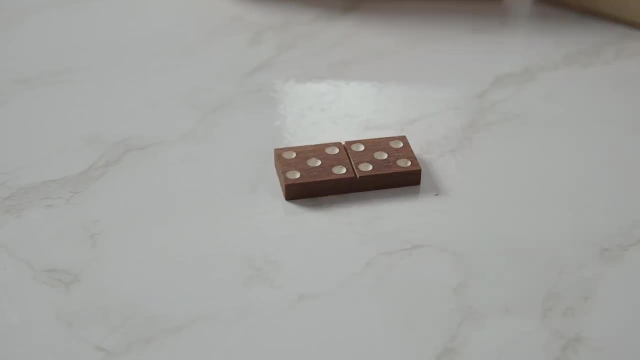 boss, Easy right. Another thing you might want to do is to set up a dominoes game. You can set up a dominoes game with a player with the highest double who lays down that domino first to start the first round. 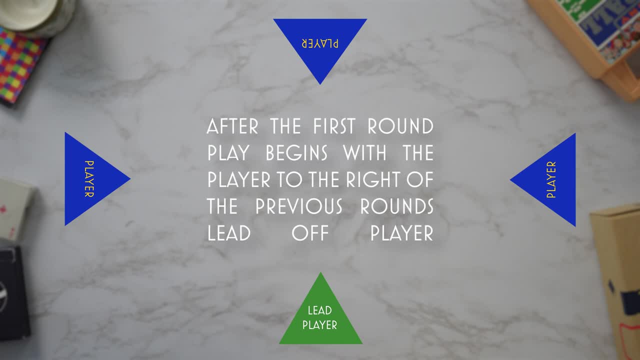 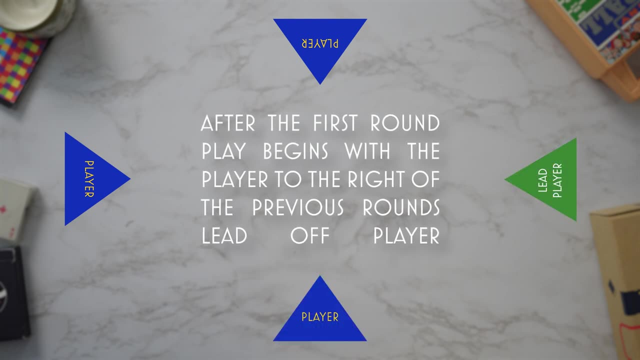 The highest double in a round is known as the heavy. Just be aware that this rule only applies to the very first round. in most plays, The next round, the player to the right gets to lead with any domino they want. I have the heaviest of the heavies, A double six, So I get to lead. 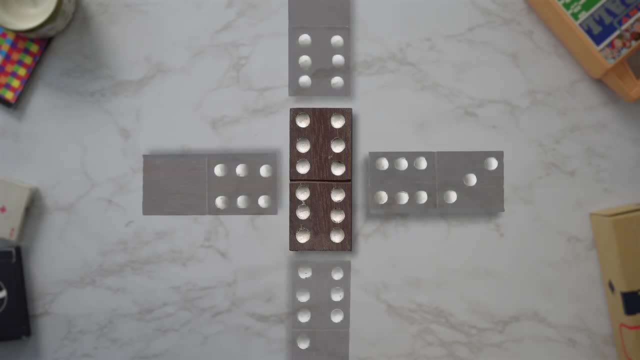 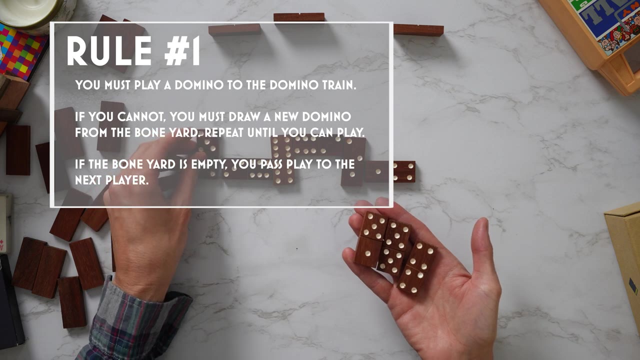 The first double domino placed down can be played on all four sides. More on that in a little bit. So here's the main rule for playing dominoes: On your turn, you must play a domino from your hand or draw more dominoes from the boneyard until you can play one. In order to play, you can only lay. 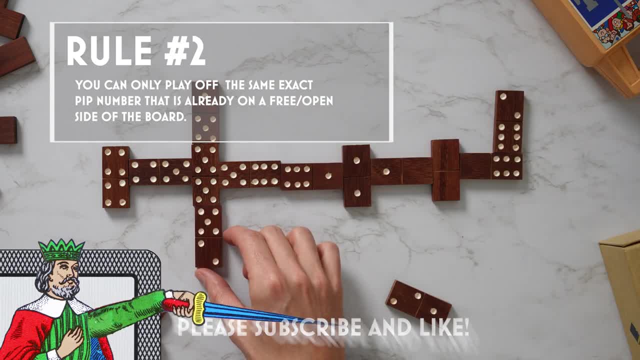 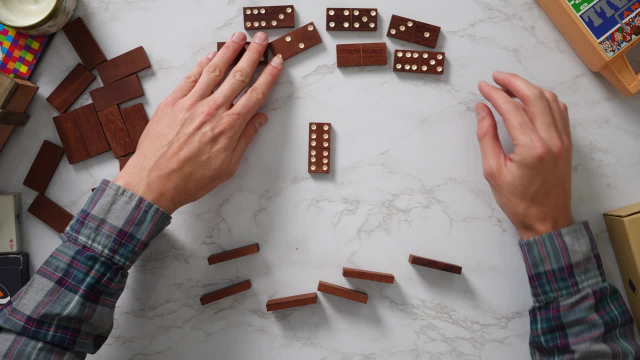 out a domino whose pip number matches an open side of the laid out dominoes: The domino train. So now the opposite player must play a domino with a pip of six. If they can't play any of the dominoes from their hand, then they must take a face down domino from the boneyard and keep taking. 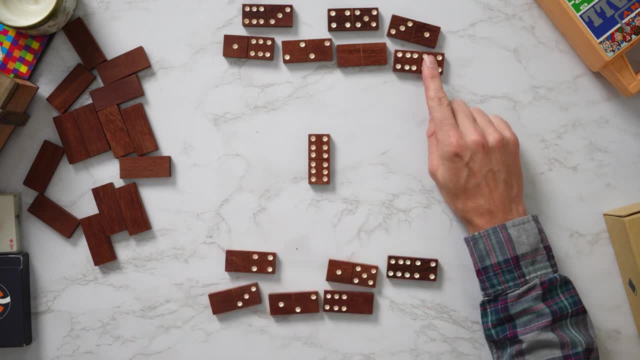 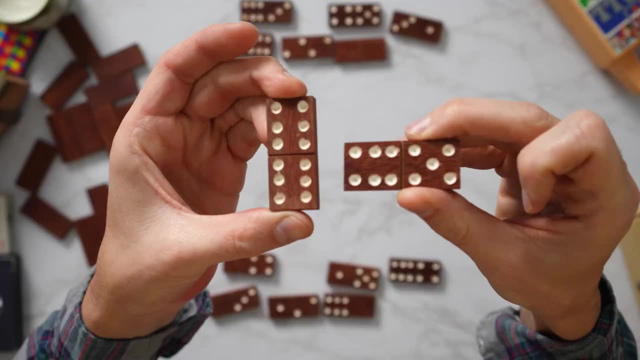 more, one at a time until they can make a play. Luckily, they have this one which shows a six and a five. When playing off a domino which has a five on the side, they can't play any of the dominoes. So if you want to play a domino which has the same number on either end, you play off these sides. 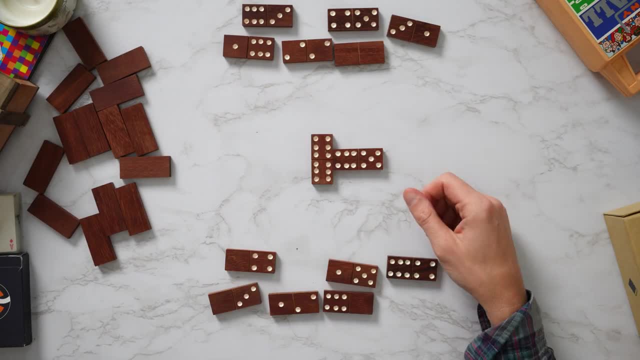 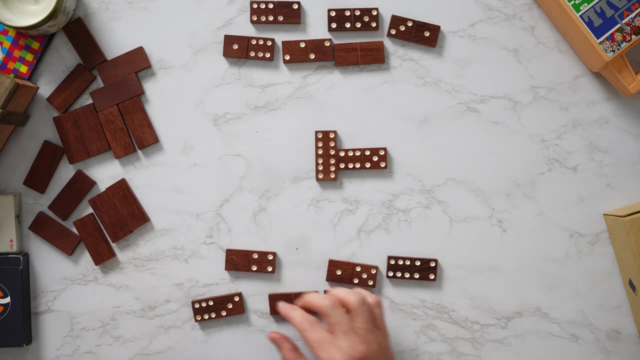 initially where the crease is And because this is the first double played, you'll be able to play off all four sides. After finishing their move, play goes to the next player. Now a six and a five are showing and I can play off either side. I'll play this domino, which has a six and a three. 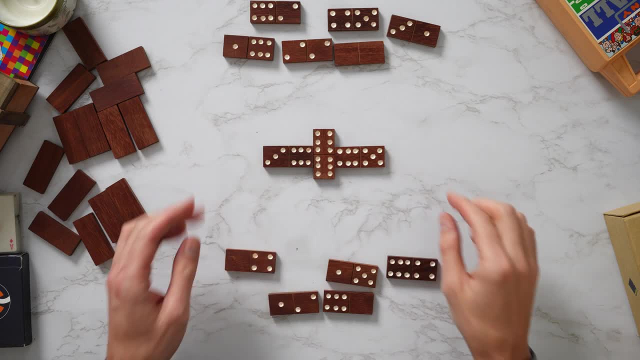 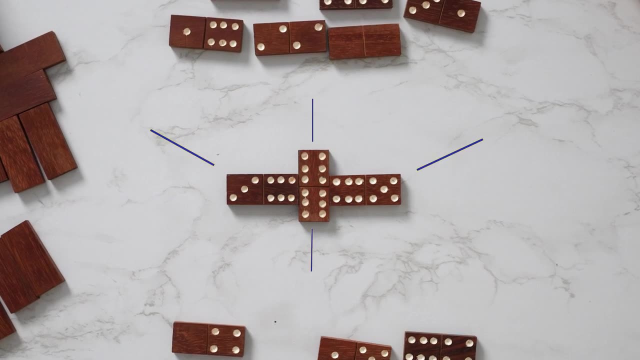 and that'll go right here. So that means the only numbers you can play off of now are the five and three, right? Actually, no, The first double played in the round can be played on all four sides. That means the next player can use a three. 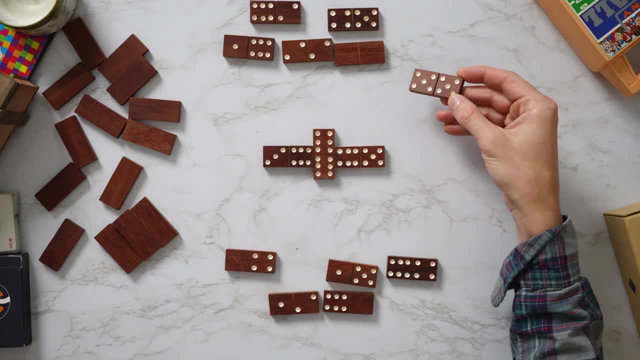 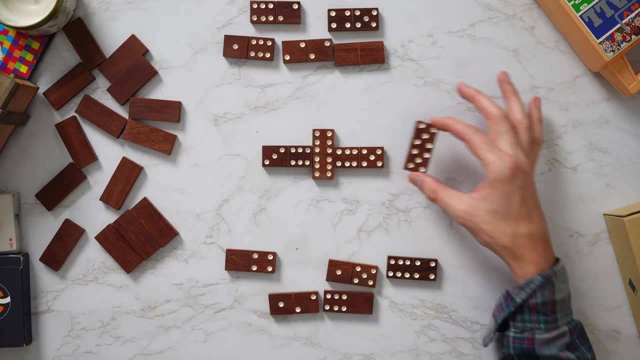 five or a six. They're going to play a double five. Now does that mean that this double five can be played on all four sides? Unfortunately, not Only the very first double can be played on all four sides, But since it's a double, it will go sideways as well. Now we continue to. 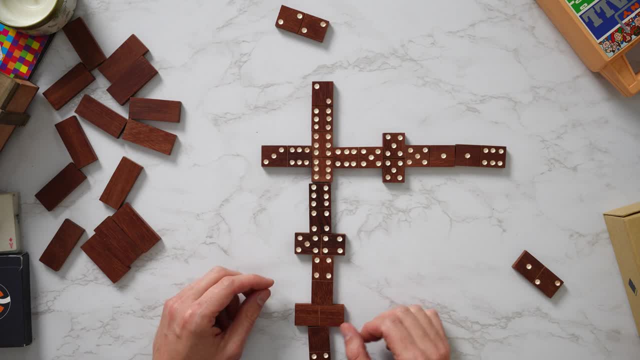 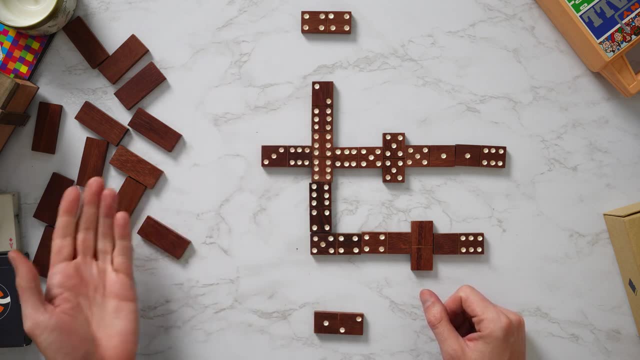 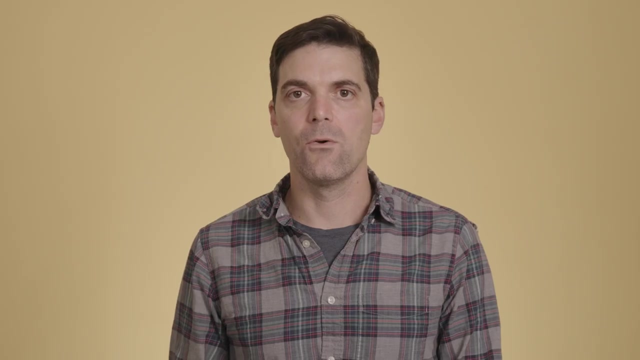 play until one of us sheds our final domino. If you run out of space, you can begin to turn the dominoes in a way that allows for more play. If a player cannot make a move, they must take a domino from the boneyard, and you'll continue to take dominoes, one at a time, until you have a domino. 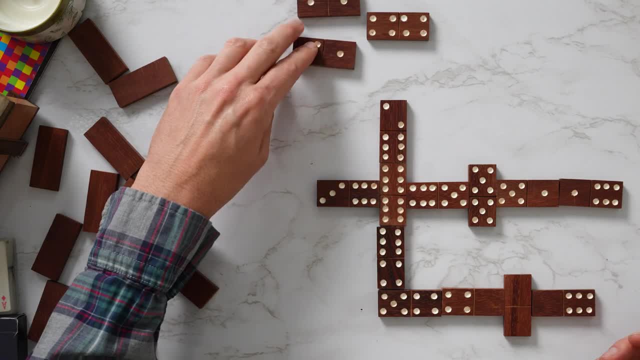 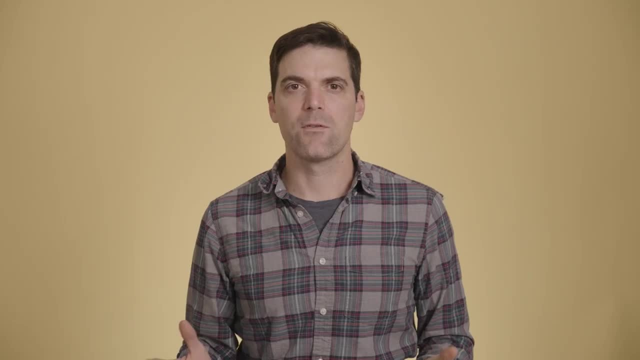 that can be played with. Okay, here's a three. I can make the last play and I'm out of dominoes. I've shed all my dominoes. I have none left. So what happens next? Well, my opponent reveals their. 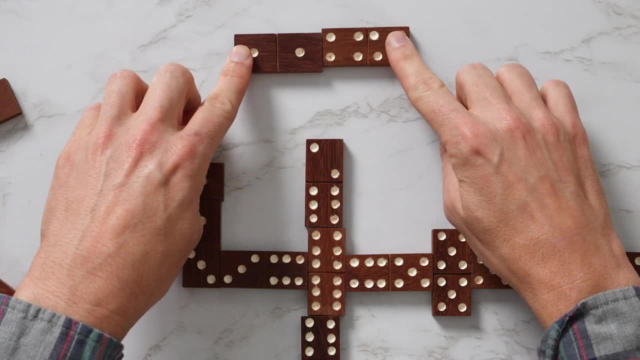 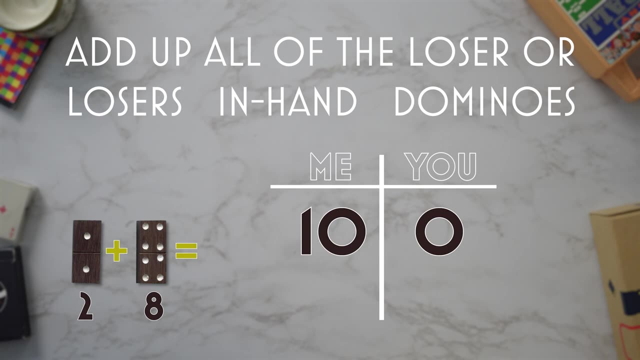 remaining dominoes, We add up all the pips and the total becomes the winner's score for that round. The opponent gets nothing. Rounds continue like this until one player has the designated final score. Here are some other tips and rules. If a player can't make a